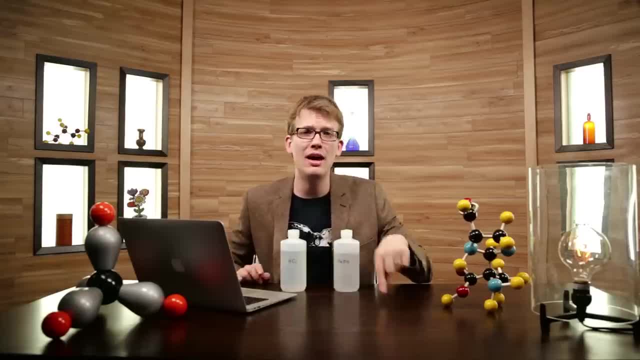 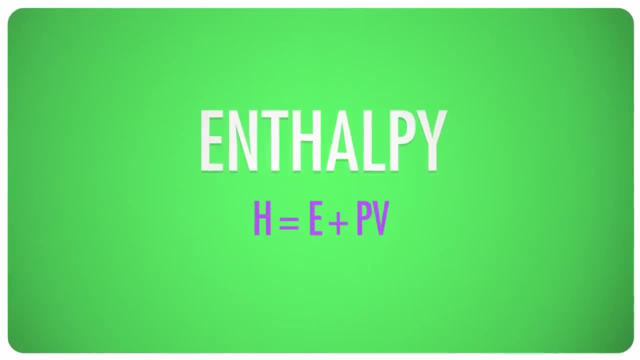 Remember that measuring heat, Heat change, is closely related to enthalpy, which we defined as the internal energy of a system, plus the energy that it uses to push the surroundings back and make room for its own pressure and volume, And at a constant pressure like we have here at the surface of the Earth. 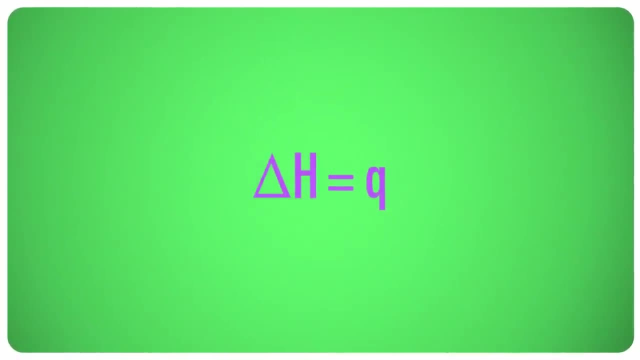 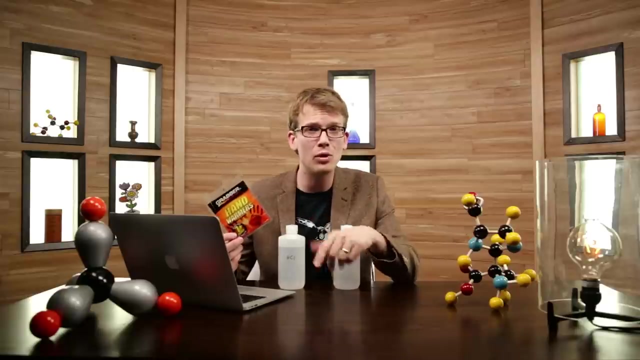 that works out to be exactly the same as the heat that's absorbed or released by a reaction. Naturally, it can be very useful to know how much heat a chemical reaction absorbs or releases. In addition to the exothermic hand warmers that we looked at, there are also endothermic chemical ice packs for treating injuries. 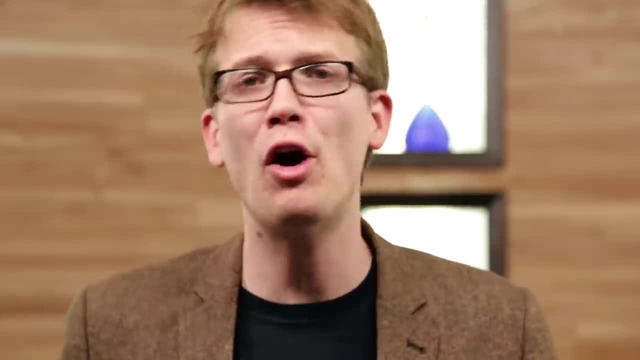 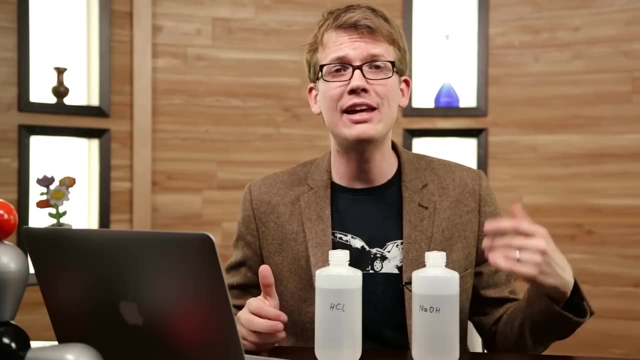 The ability to calculate change in enthalpy is also what tells pilots how far the fuel in an airplane's tank will allow it to fly, which I am personally very interested in making sure they get right. One of the ways we can calculate the change in enthalpy of a system is with Hess's Law. 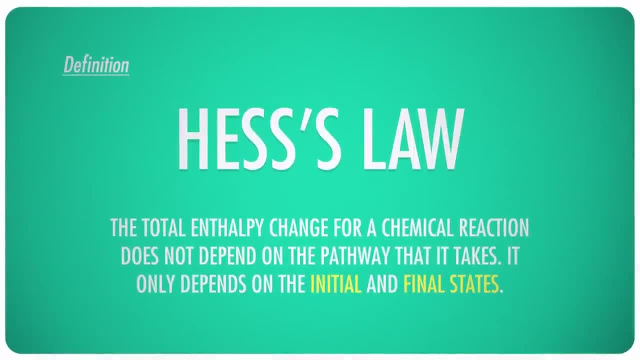 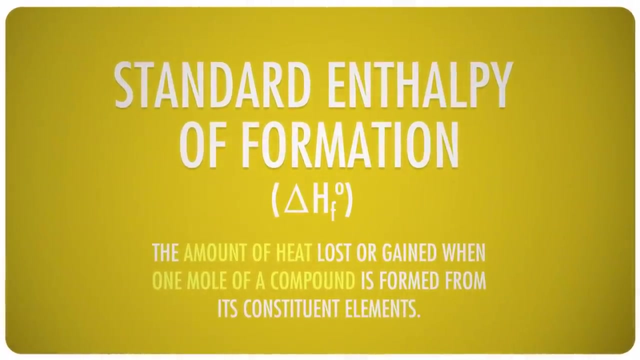 which, you'll recall, states that the total enthalpy change for a chemical reaction doesn't depend on what pathway it takes, but only on its initial and final states. It's often expressed in terms of standard enthalpies of formation, that is, the amount of heat lost or gained when one mole of a compound is formed from its elements. 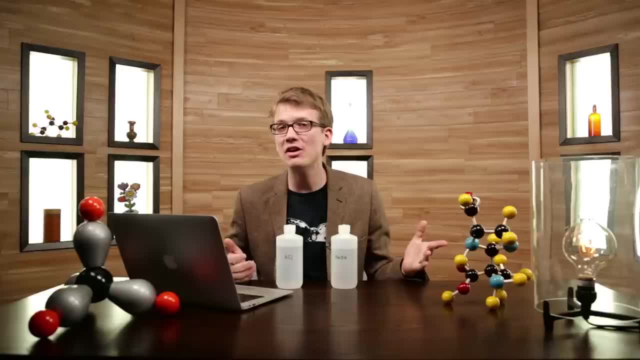 That's how we figured out exactly how much heat a chemical reaction absorbs and how much heat my hand warmers release. But that's not the only way that Hess's Law can be used. The law itself says nothing about standard enthalpies of formation. 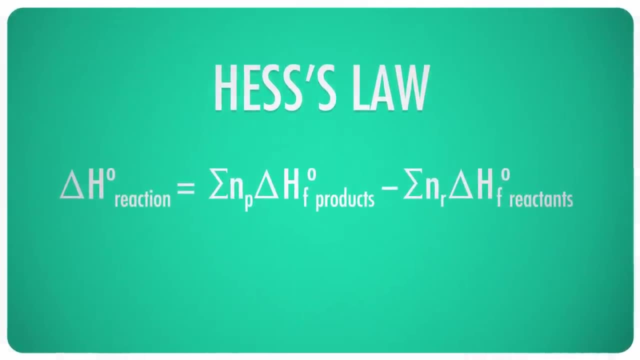 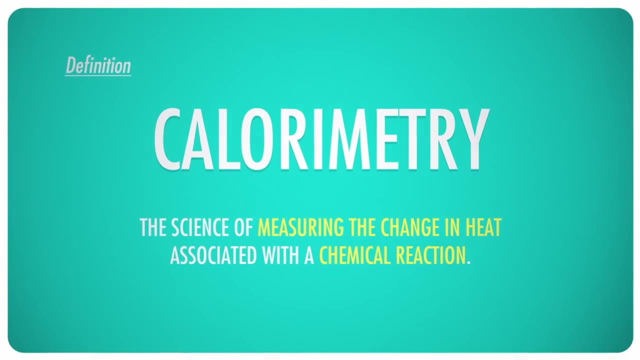 Any way that we can figure out the change in heat between the products and the reactants will work just as well. And that's where calorimetry comes in. Calorimetry is the science of measuring the change in heat associated with a chemical reaction. 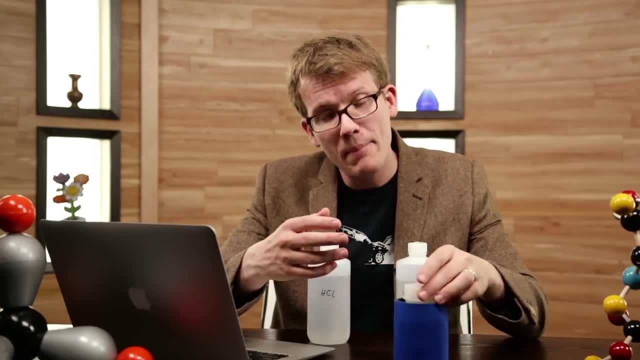 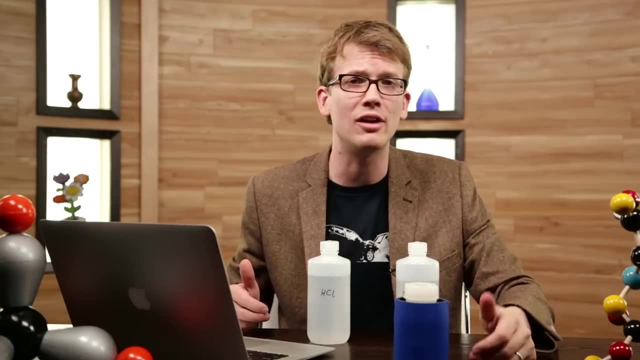 And this may look like a plastic bottle inside of a koozie, but it's actually a calorimeter. A calorimeter can be a fancy and expensive piece of hardware or it can be simple, But no matter what it looks like, it's basically just an insulated container that contains a thermometer. 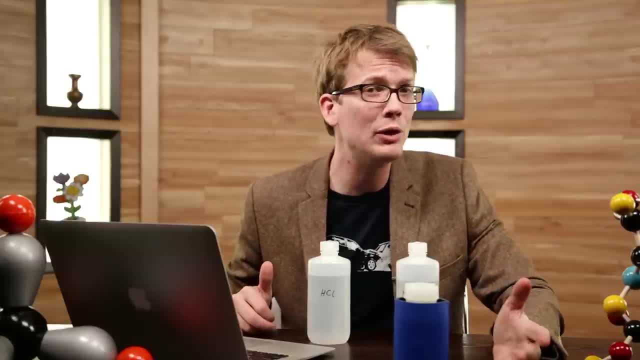 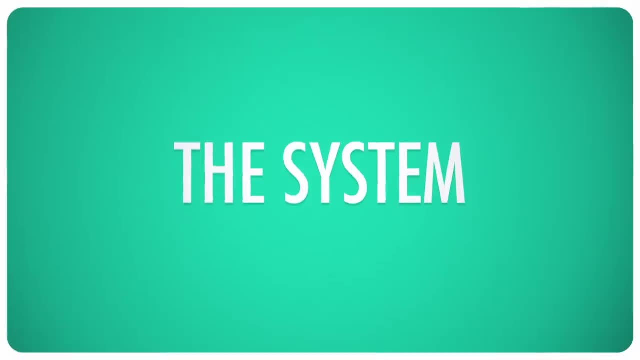 And it can be made out of stainless steel or styrofoam cups, but there really are no fundamental differences in how they work And you know the general setup by now. The chemicals in the calorimeter make up the thermodynamic system and everything else is the surroundings. 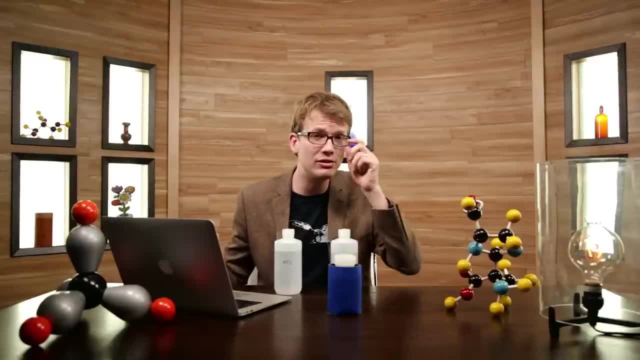 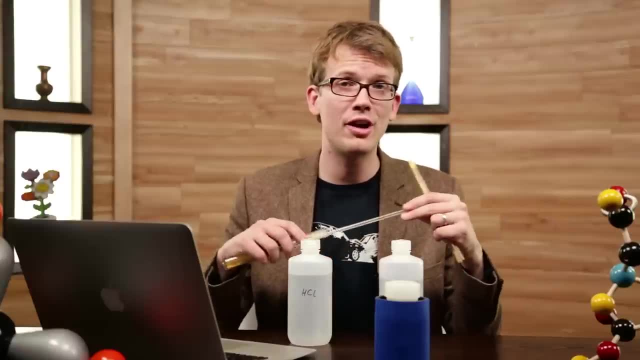 The insulation minimizes the amount of heat that leaks in or out of the system, so that we can be fairly confident that any heat transfer is part of the system, not the surroundings. The thermometer tracks the temperature change, which is part of the calculation we have to do. 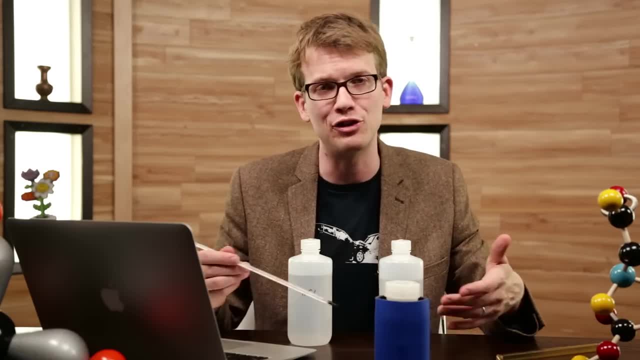 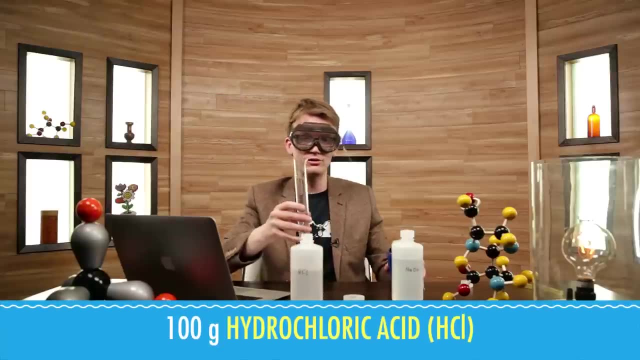 And there's usually some way to stir the solution to make sure that the reaction occurs fully. All right, everybody. Safety first, though I really should be wearing gloves. I'm going to put 100 milliliters, also 100 grams. 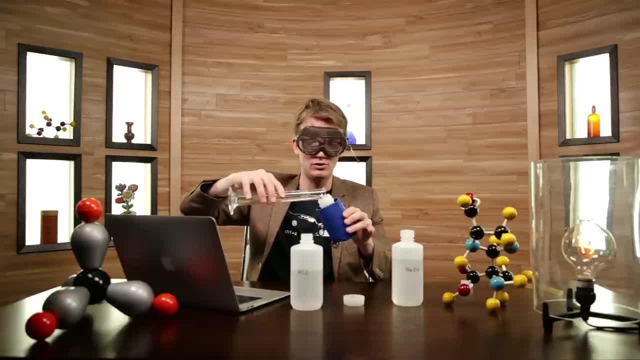 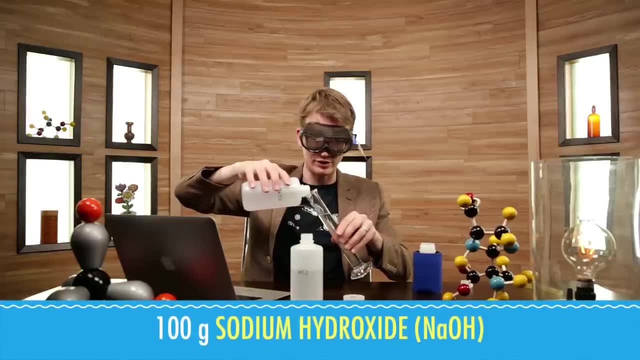 of HCl's, one molar HCl solution into my calorimeter. here I'll wash it up, And now I'm going to put the same amount of sodium hydroxide solution. Before I do the reaction, I have to know our starting temperature. 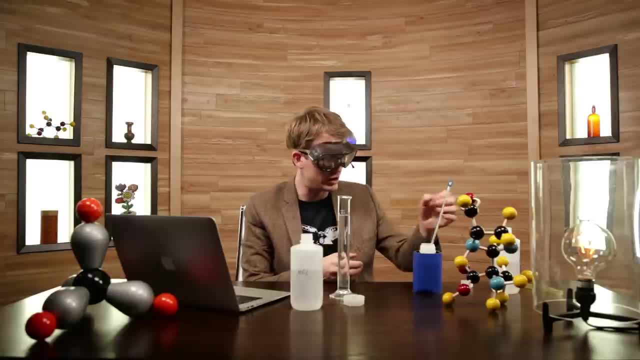 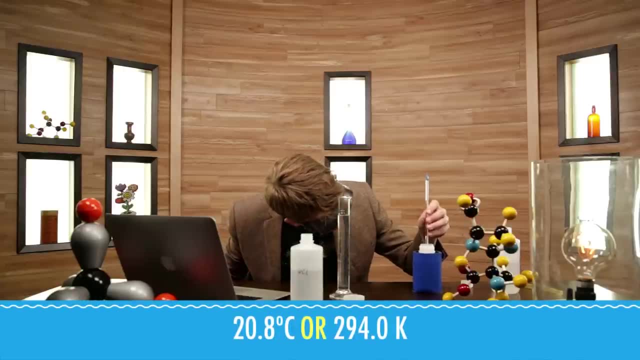 so I'm going to stick my thermometer in there and wait for a second To see what it does. It should be roughly room temperature. It's been in the room for a long time, So we are currently at like 20.8 degrees Celsius. 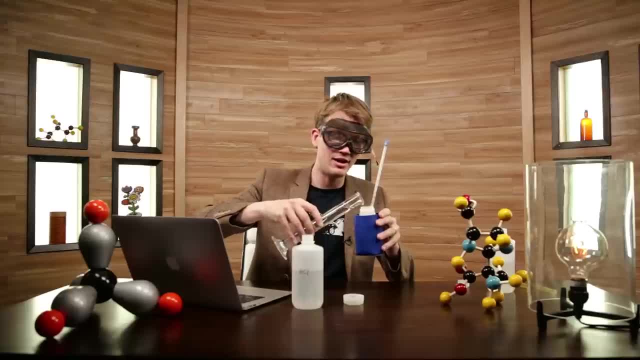 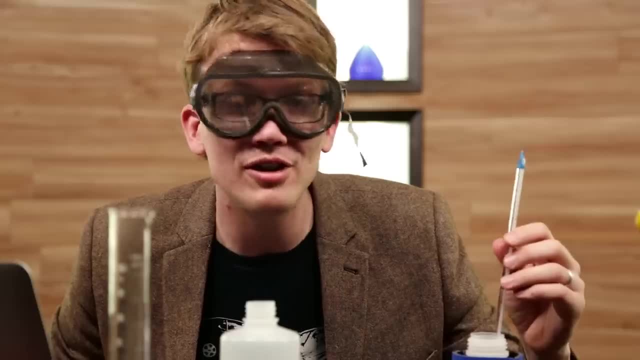 So that's like 294 Kelvin, And now I shall add my 100 milliliters of sodium hydroxide. The temperature, unsurprisingly, is rising very rapidly, And I'm doing something right now that you should never, ever do, which is stir with the thermometer. 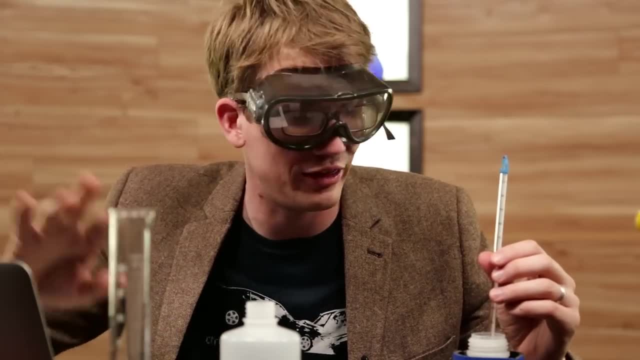 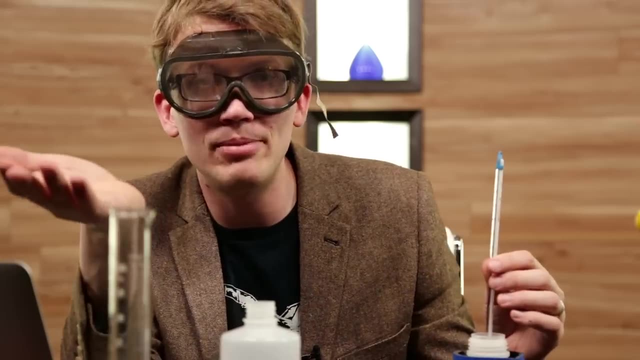 Because If this happens in schools across the world, then there will be a million billion broken thermometers and the stuff inside these thermometers is not good. So never do what I'm doing. Alright, the temperature should be stable by now. 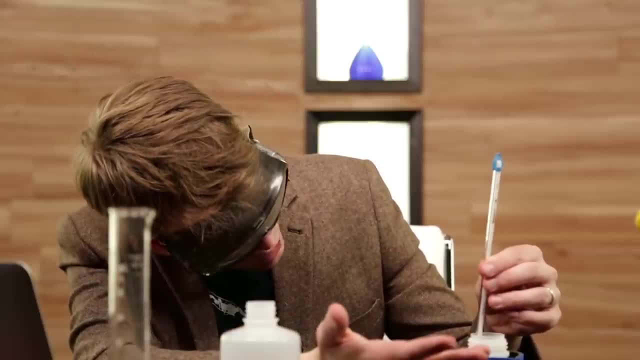 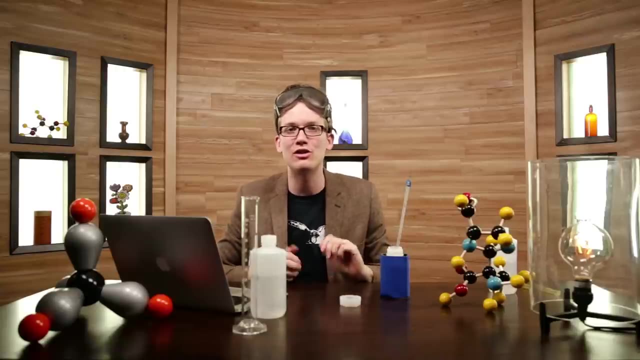 We have 28.2 degrees Celsius. Now there's a simple formula that allows us to calculate the heat change of a reaction simply by measuring the change in temperature that occurs in a calorimeter. It says that the change in heat equals the specific heat capacity of the substance. 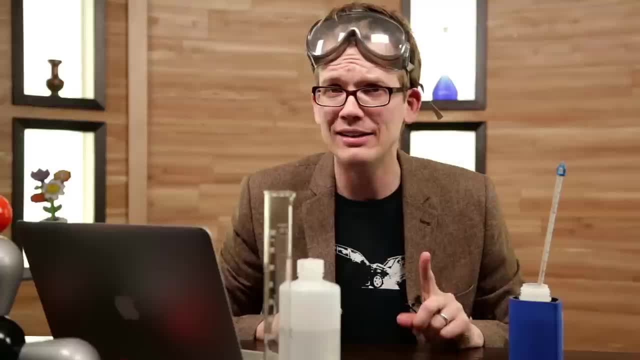 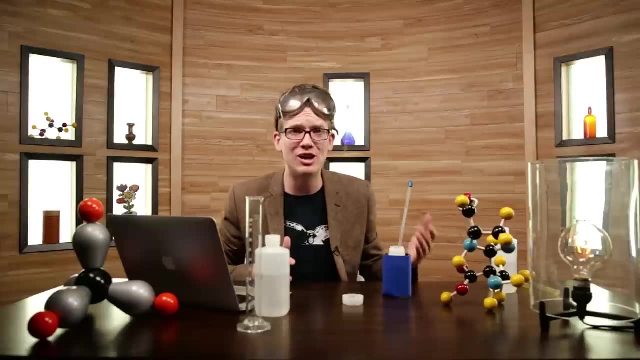 times its total mass, times the change in temperature. Let's examine the parts of this. First of all, the heat change in the calorimeter formula is normally represented by a lowercase q, but it can also be represented by change in enthalpy or delta H. 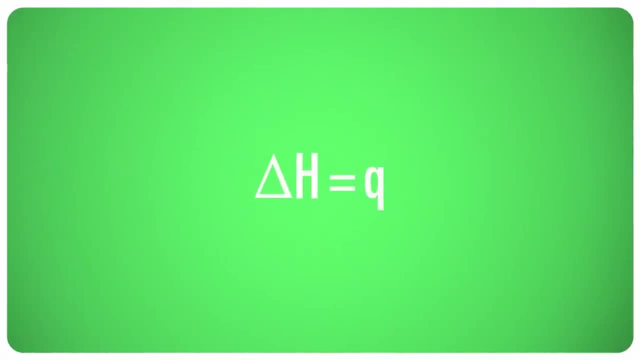 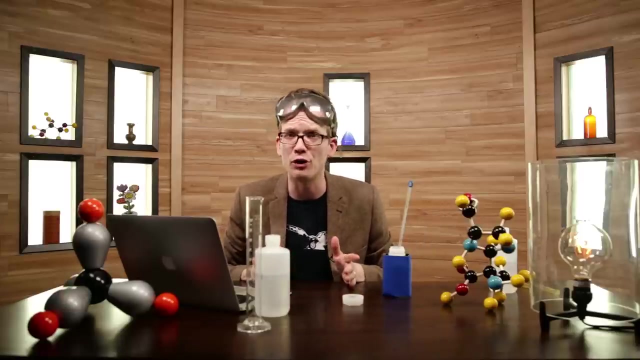 because, remember, at constant pressure delta H equals Q, And constant pressure is almost always a good assumption for the duration of an experiment, or at least as long as we stay at the surface of the Earth, For reasons that will become clear later. 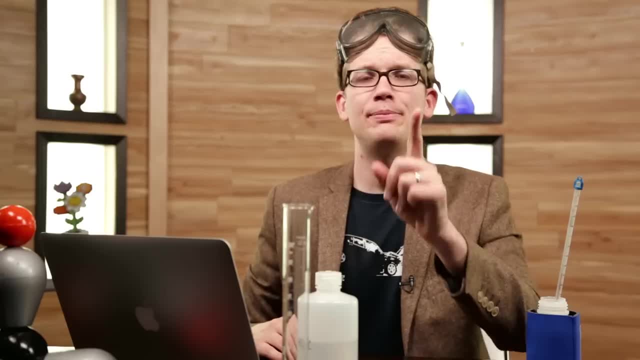 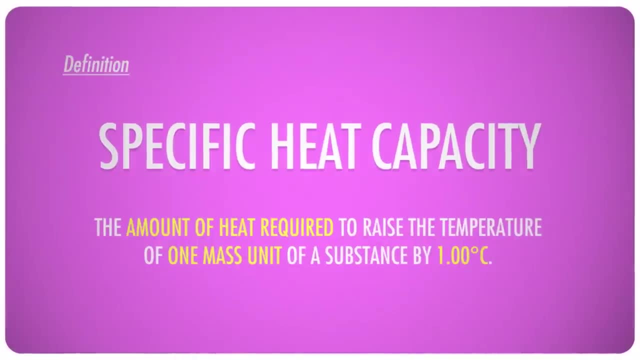 we'll use delta H to represent the heat change for this experiment. Specific heat capacity, represented by a lowercase s, is the amount of heat that is produced in the experiment. This is the amount of heat required to raise the temperature of one mass unit. 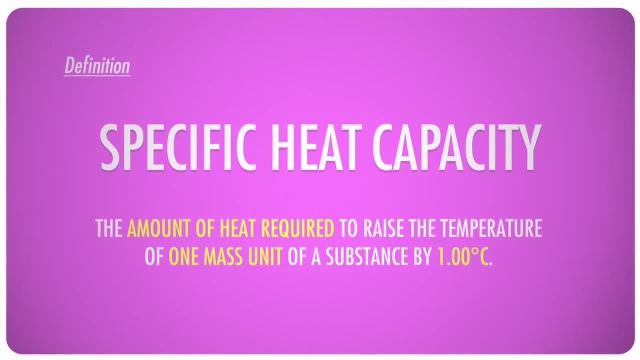 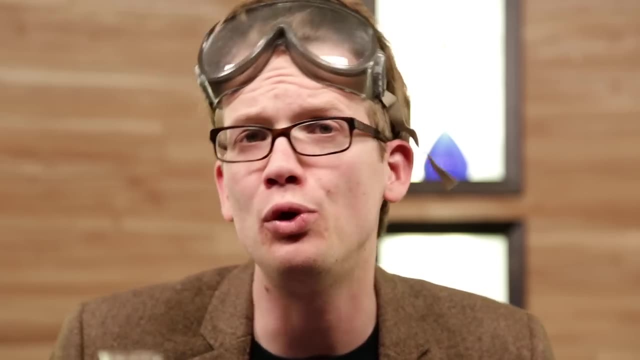 like a gram or kilogram of a substance by one degree Celsius. So it turns out that different amounts of heat create different temperature changes. like metals get hot really easily and cool down really easily. Others, like water, require a lot of thermal energy to raise the temperature. 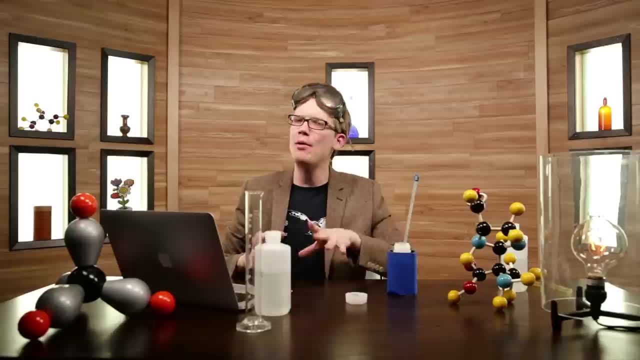 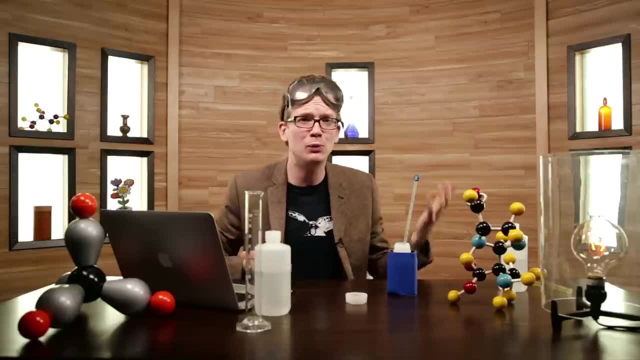 and therefore have to release a lot of heat to cool down. I'm always wondering, though: like what does that really mean? Like physically in the molecules, shouldn't heat raise the temperature of all substances equally, And why does water in particular have such a high specific heat capacity? 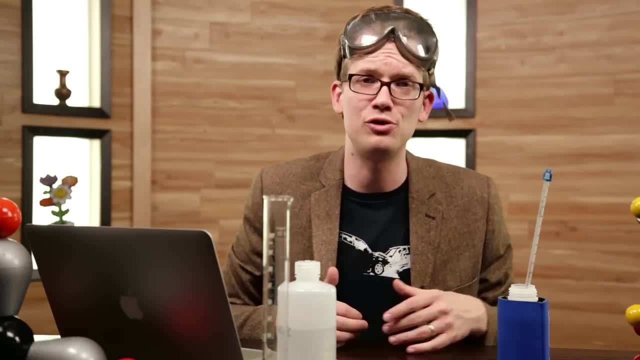 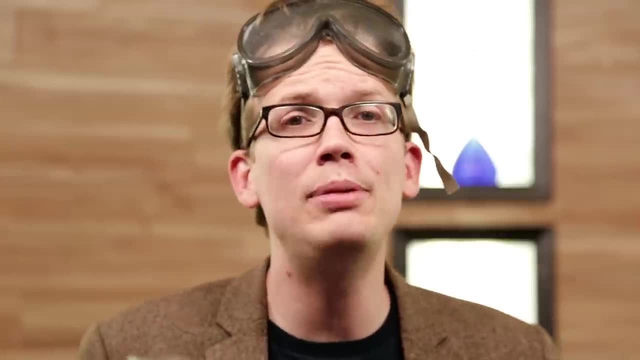 Heat energy can do a lot of things besides just increase temperatures. Temperature, or the speed at which molecules bounce around, is just one way that atoms or molecules can absorb energy. Heat energy can also be absorbed by the breaking and formation of bonds between molecules. 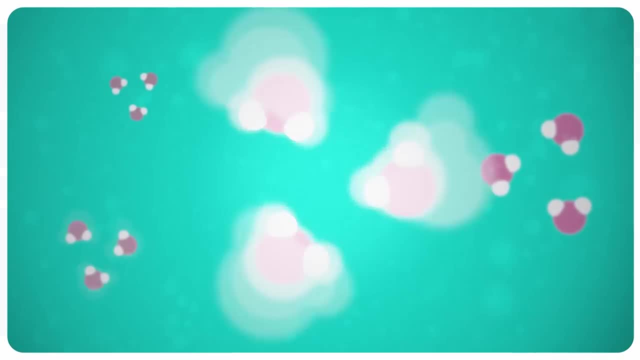 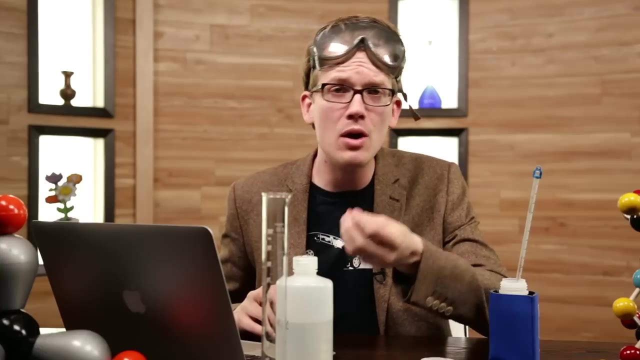 And, as we'll learn in another episode, the extremely high specific heat capacity of water is due to the breaking and formation of hydrogen bonds that are associated with relatively small changes in temperature. And how do we know The specific heat capacity? Well, I am happy to report that some noble chemists have worked hard to determine the 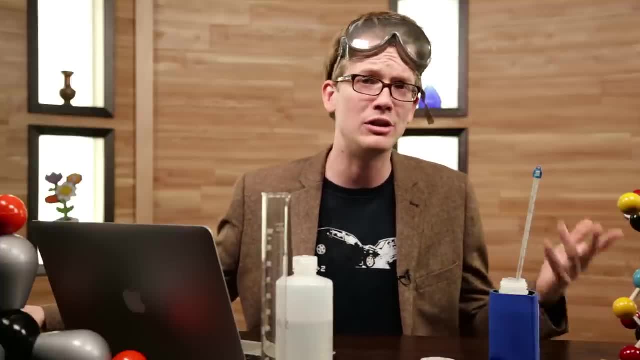 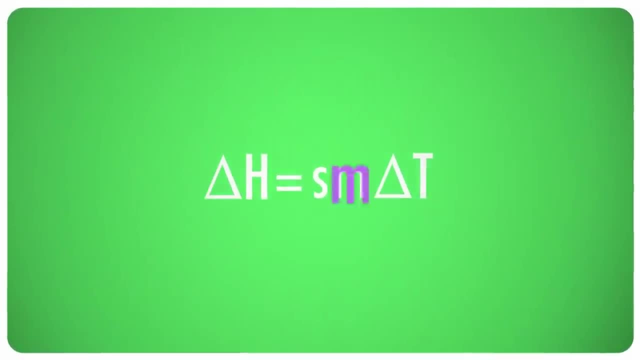 specific heat capacities of hundreds of substances, so that we don't have to, We just have to look up the numbers in a table. Okay, so specific heat capacity times, mass times, the change in temperature. The mass is important because the more mass of a substance we have, 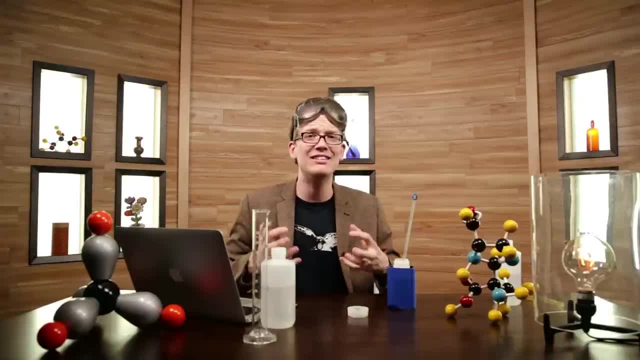 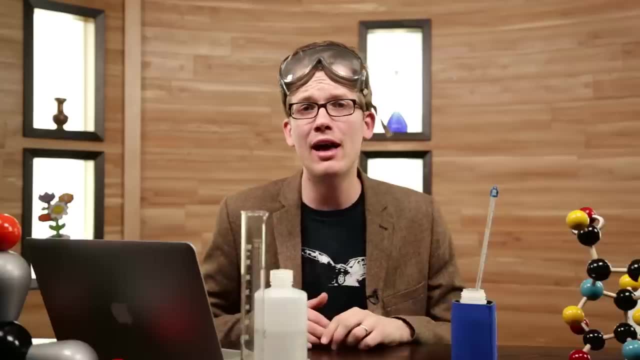 the more chemical bonds are present, And because energy is contained in chemical bonds, they have a big effect on how much energy we're able to absorb or release. And finally, there's the change in temperature. When doing calorimetry, we calculate a change in heat by measuring a change in temperature. 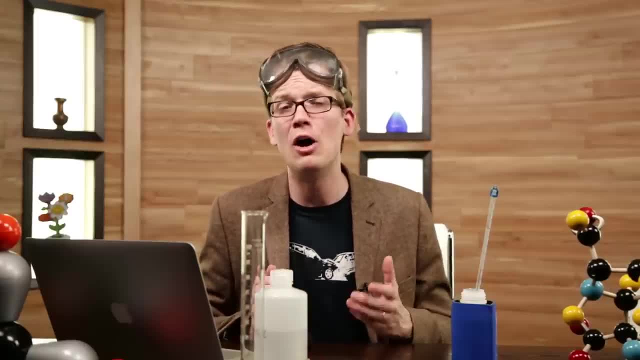 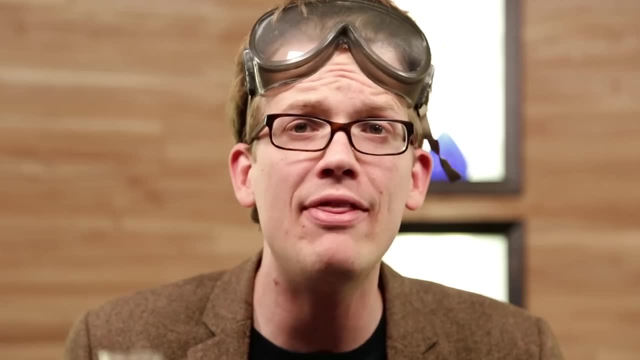 But, as we've said a billion times before, heat and temperature are not the same thing. Please do not think that this thing is measuring heat, because it's not. It's just that, luckily, in this specific case, they are related by our handy little calorimeter formula. 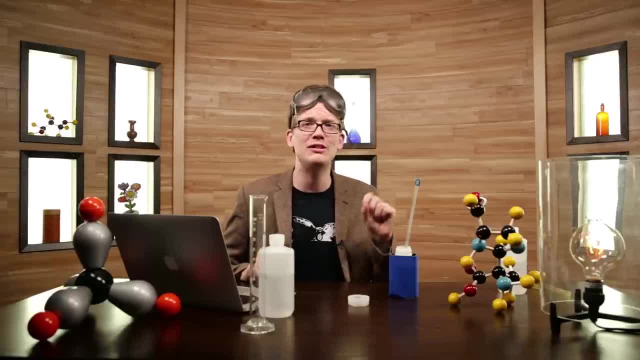 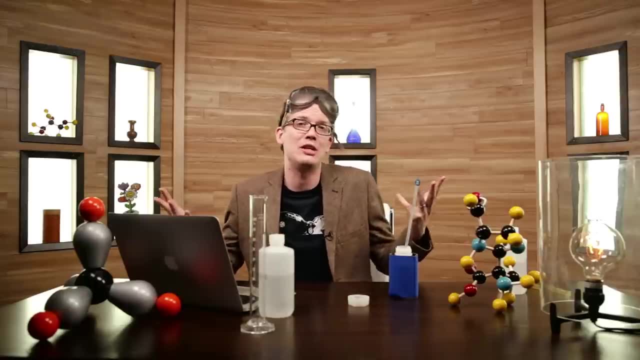 Now you might not have noticed, but we are right at the interface between chemistry and physics here. Each science could claim ownership over these phenomena, but the truth is that humans made up the difference between chemistry and physics anyway. Thermodynamics: the study of heat, energy and work. 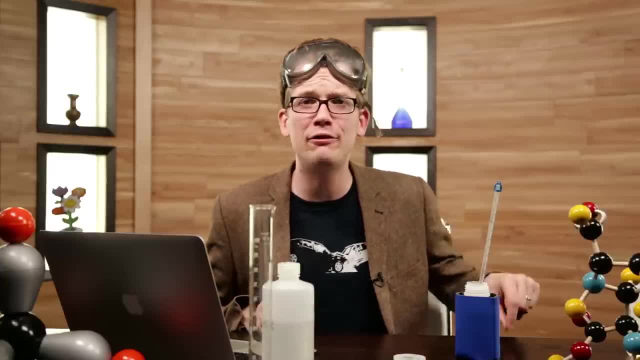 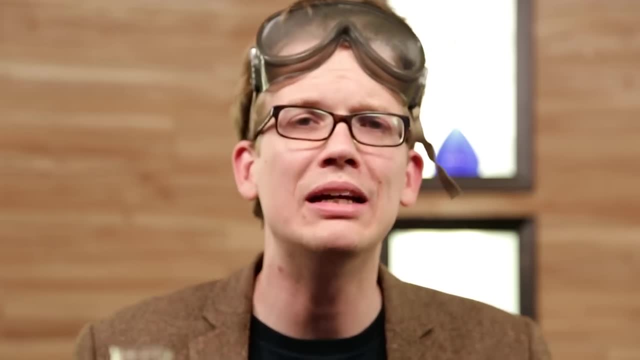 doesn't care about our little rules. Thermodynamics itself makes the rules of the universe. It is the ultimate law. So now you know, even though you might not have cared, but you should, because it's cool. It's all wiggly, wobbly, bondy-wandy. 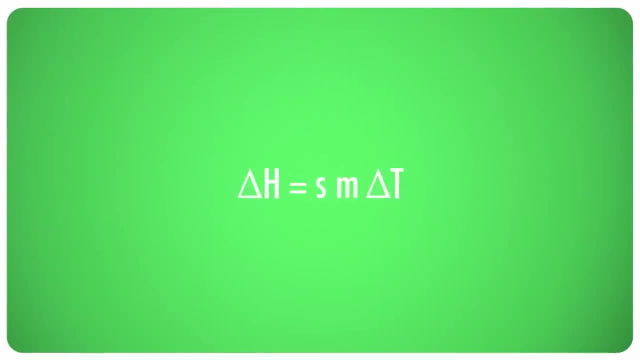 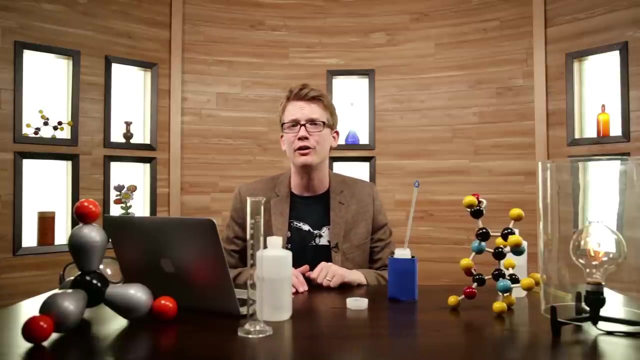 All right, enough talk, Let's get out there. I actually do some math here. Remember that the formula is delta H, S M, delta T. The solutions we're using here are so dilute that almost all of their mass consists of water. 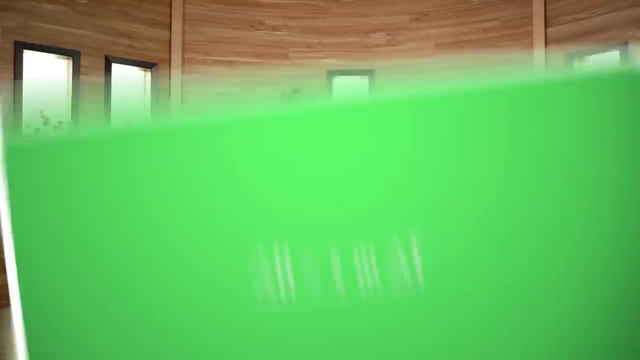 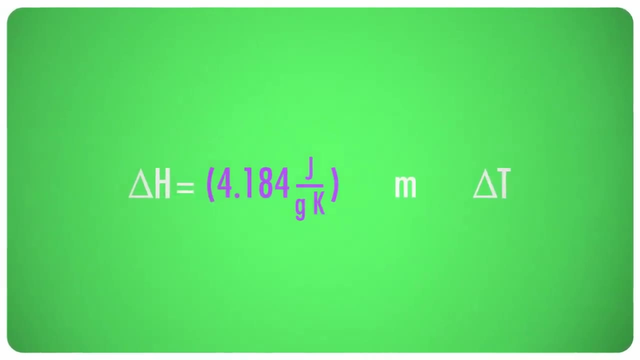 Therefore, we can simply use this formula. We can use the specific heat capacity of water. If we look that up on a table, we'll see that it is 4.184 joule per gram degree Celsius. I used 100 grams of each chemical for a total mass of 200 grams. 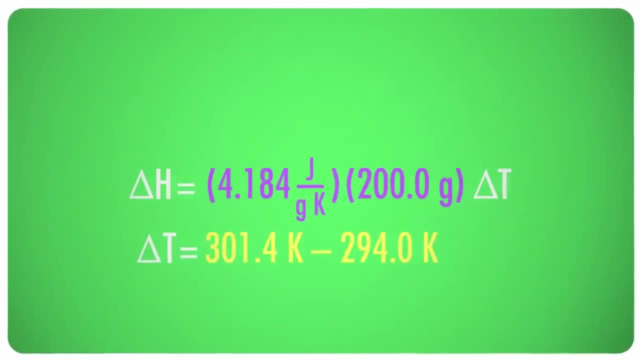 And finally, we need the temperature change. If you remember, the temperature rose from 294 Kelvin to 301.4 Kelvin. The difference between these two is 7.4 Kelvin. It's a positive value because the temperature increased. Cancel all the appropriate units and then bang on the calculator. 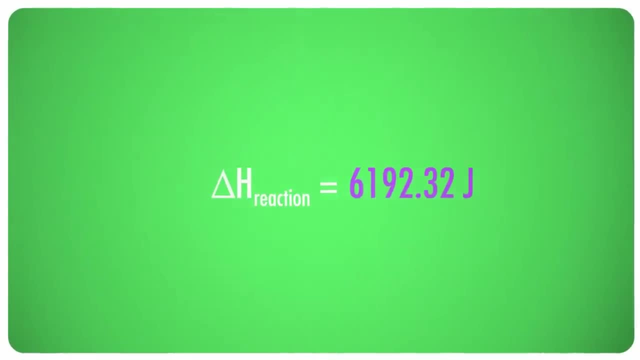 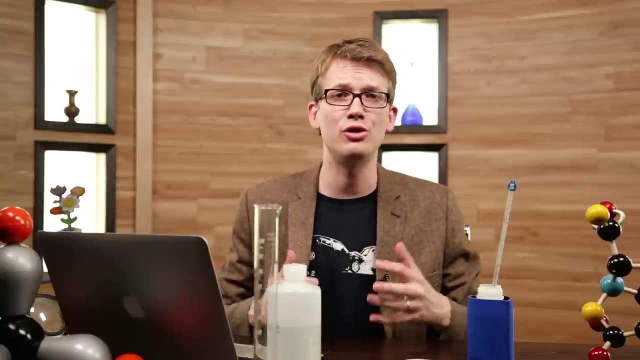 to get a final release of 6192.32 joules- 6.2 kilojoules- of heat from the reaction, Because this formula is based on temperature change and since the temperature increased, we end up with a positive result. 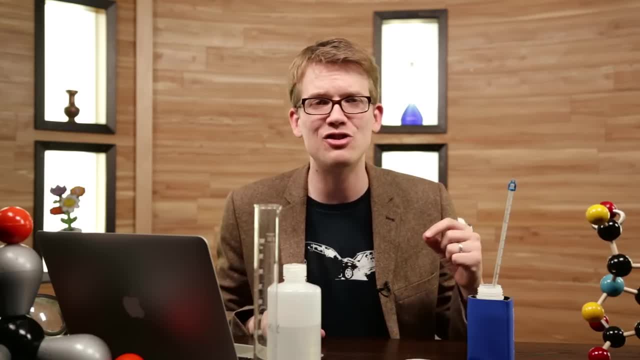 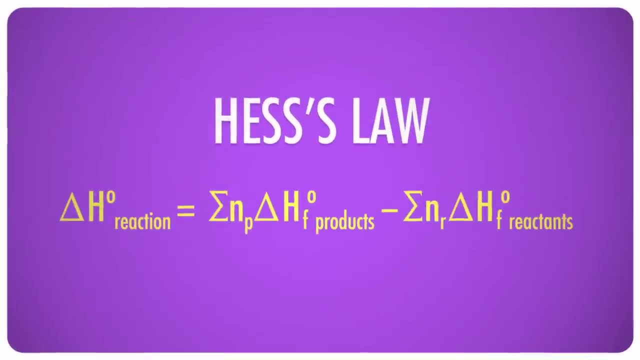 But most importantly, it tells us the magnitude of the change in heat energy. So I wonder how that compares to the amount we would predict using Hess's law and the standard enthalpies of formation. Remember that we can look up the standard enthalpies of formation. 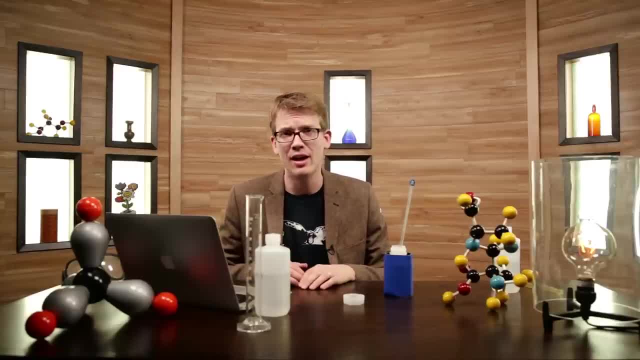 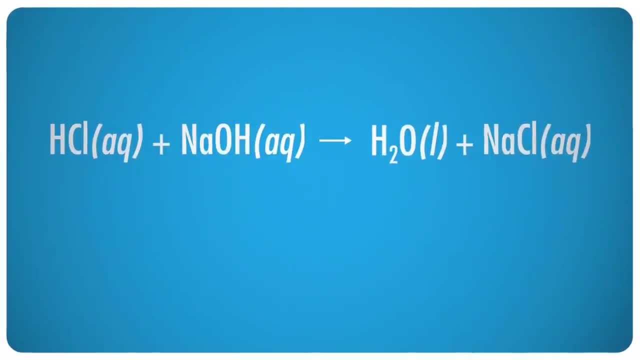 for all the products and reactants in the back of a textbook or online. The chemical reaction between hydrochloric acid and sodium hydroxide produces liquid water and sodium chloride. The standard enthalpy of formation for hydrochloric acid is negative: 167.2 kilojoules per mole. 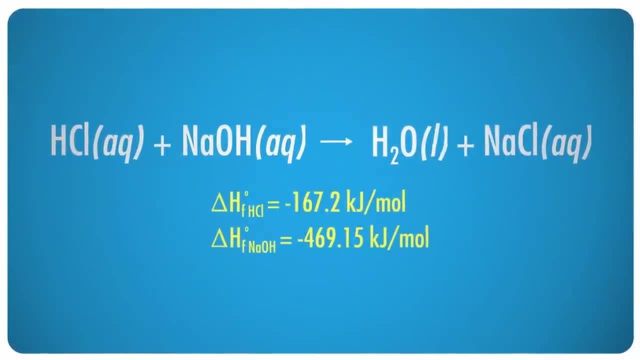 For sodium hydroxide it's negative: 469.15 kilojoules per mole. For liquid water, negative 285.8.. And for sodium chloride, negative 407.27.. I'm not going to do the mole calculations on screen. 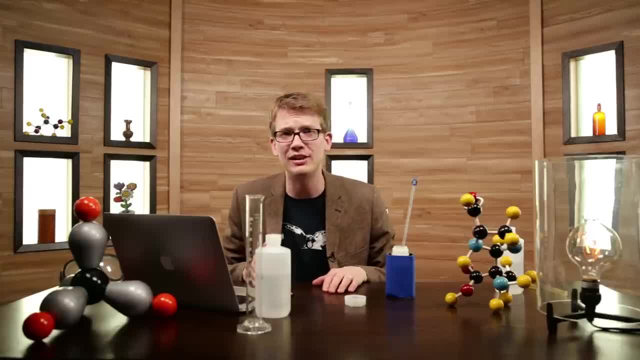 but trust me when I say that we used 0.100 mole of HCl and the same amount of NaOH, Because everything in the equation balances. it's just a 1 to 1 to 1 to 1 ratio. we can assume that they all have the same amount of each product as well. 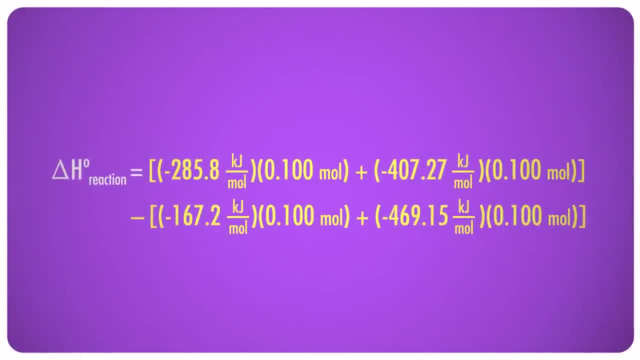 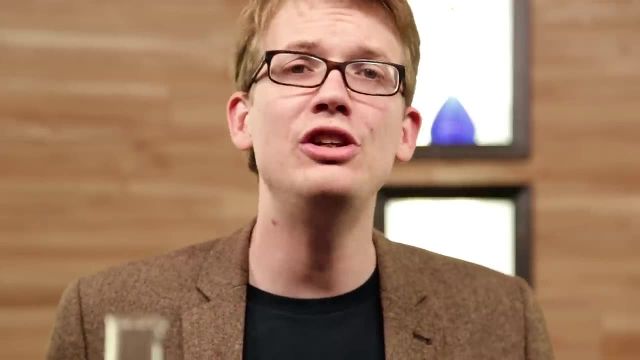 If we plug these into Hess's law and do the calculation, we find that the change in heat or enthalpy of the reaction is negative, 5.67 kilojoules. The system is releasing or losing energy, so the number is negative. 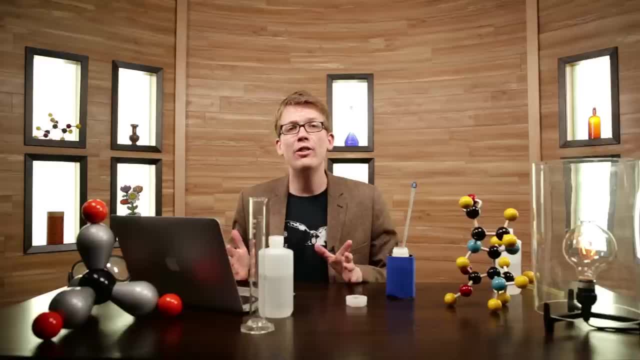 But again, it's really the magnitude that we want to know. So there you go. The calorimetry formula gave an absolute enthalpy change of 6.2 kilojoules, while Hess's law gives a change of 5.67 kilojoules. 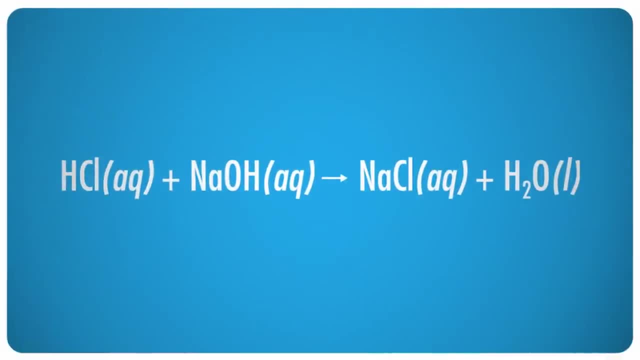 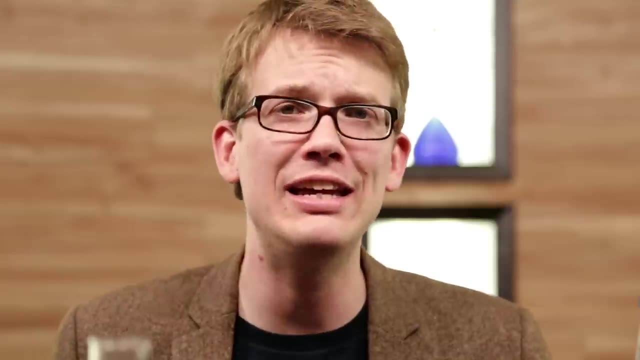 So why the difference? Well, the greatest factor is probably that we used the specific heat capacity of pure water instead of the salt water that we actually created. We also didn't include the heat capacity of our calorimeter itself. The calorimeter walls and the thermometer were heated too. 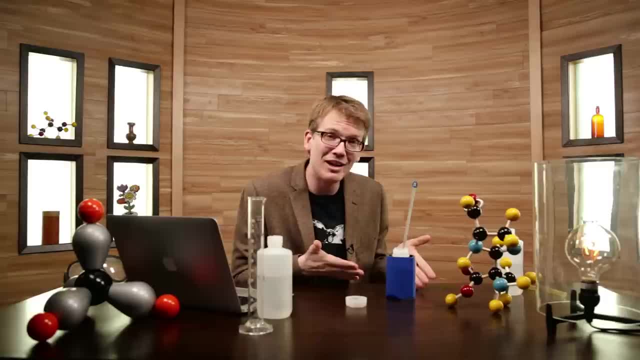 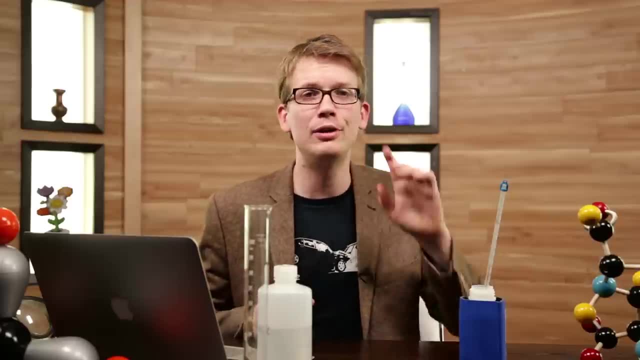 resulting in some of the produced heat not being accounted for. The insulation of the calorimeter is obviously a bit light, which allowed some heat to escape entirely, and that's another major factor. Even so, I'd say we did pretty well. The important thing is that it showed us what we needed to see. 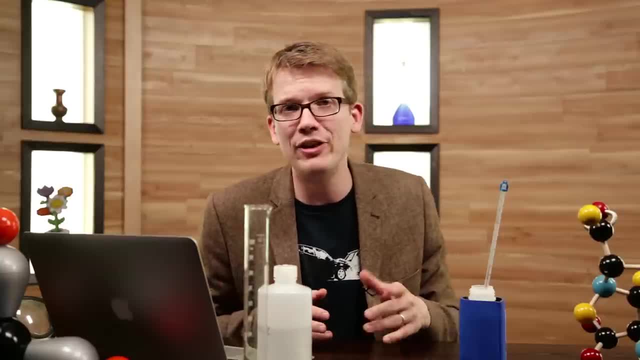 even though it was just a little plastic bottle in a koozie For a quick, simple method, the calorimeter got us pretty close to the calculated value. If we were calculating the amount of a particular fuel that we would need to travel to Mars. 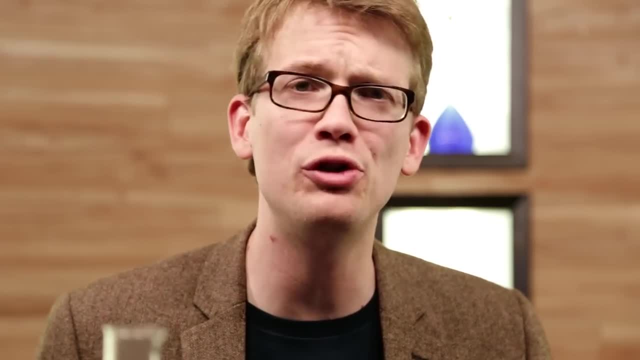 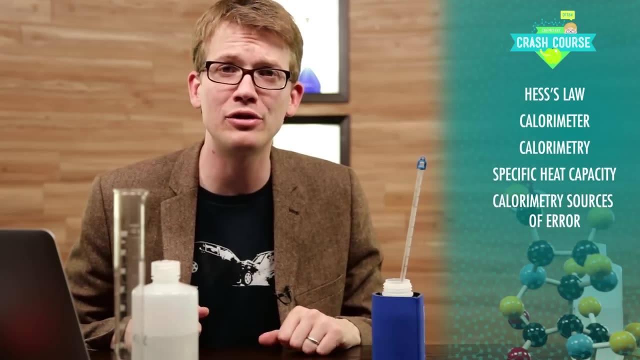 or inventing a cold pack that won't give you frostbite. we'd want to use a more sophisticated system and work more carefully, But this one's pretty cool for our purposes. Thanks for watching this episode of Crash Course. If you've hit attention. 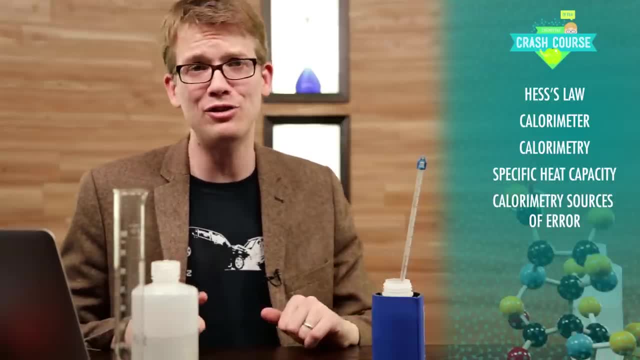 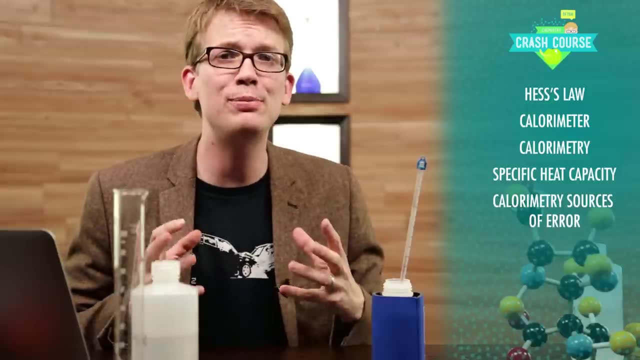 you learned that we don't necessarily have to use standard enthalpies of formation to solve Hess's law. You learned what a calorimeter is, that calorimetry is another way to investigate heat changes and chemical reactions, and that specific heat capacity tells us how much heat energy affects the molecules in a substance. 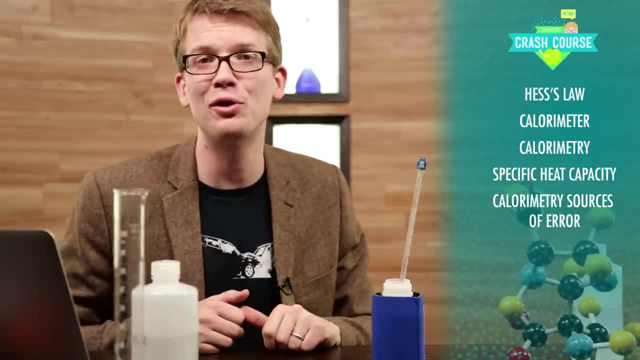 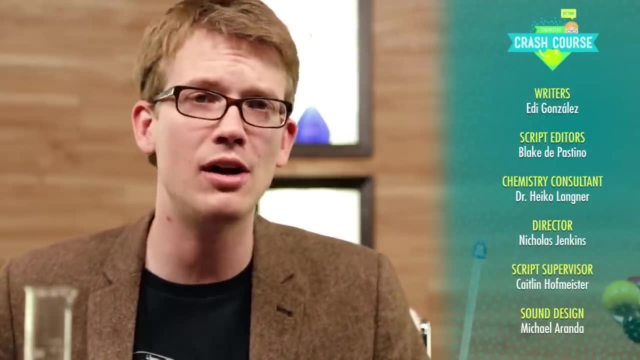 without changing its temperature. And finally, you learned some potential sources of error related to calorimetry. This episode of Crash Course Chemistry was written by ED Gonzalez, the script was edited by Blake DePastino and our chemistry consultant was Dr Heiko Langner. 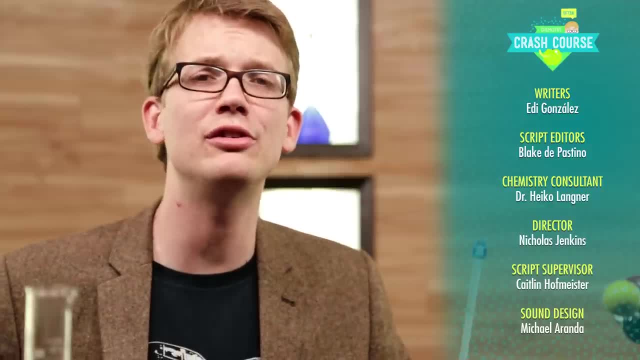 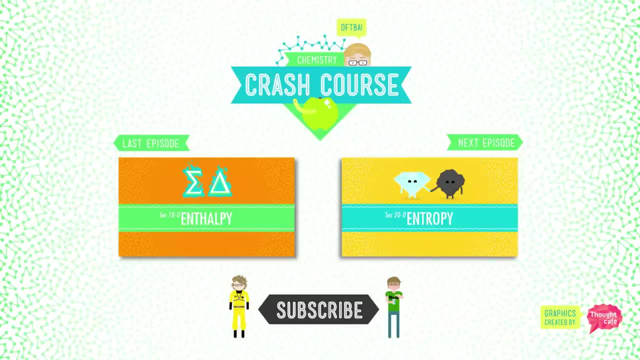 It was filmed, edited and directed by Nicholas Jenkins, our script supervisor is Caitlin Hoffmeister and our sound designer is Michael Aranda, And, of course, our graphics team is Thought Cafe. Thanks for watching.